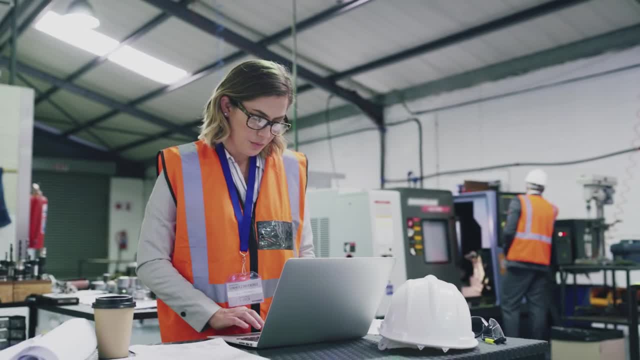 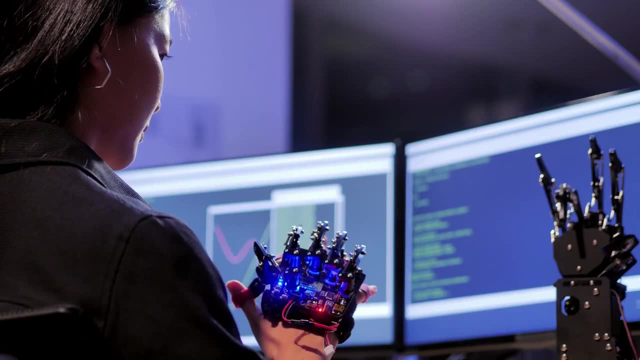 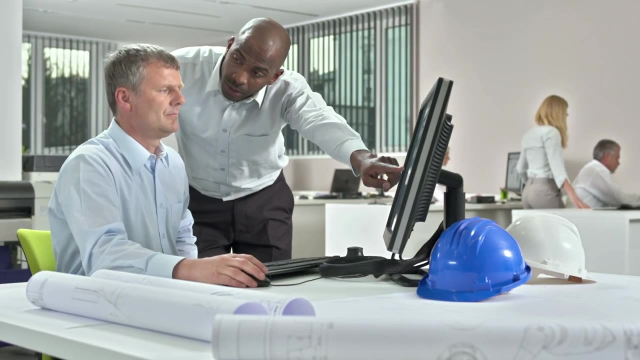 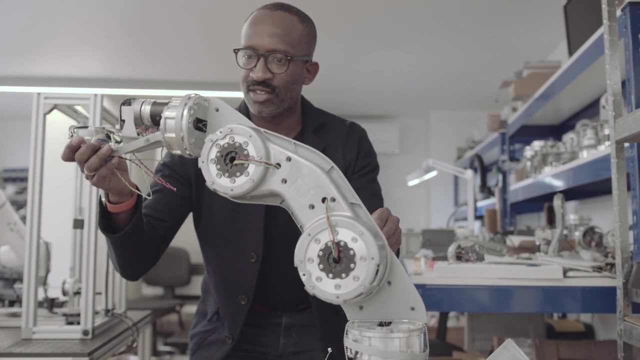 The science, technology, engineering and mathematics career cluster offers opportunities for inventive, science- and data-loving minds to solve complex problems for a wide variety of products and industries. While the majority of STEM occupations require a four-year degree, the four STEM sectors differ both in types of career options and projected job openings. 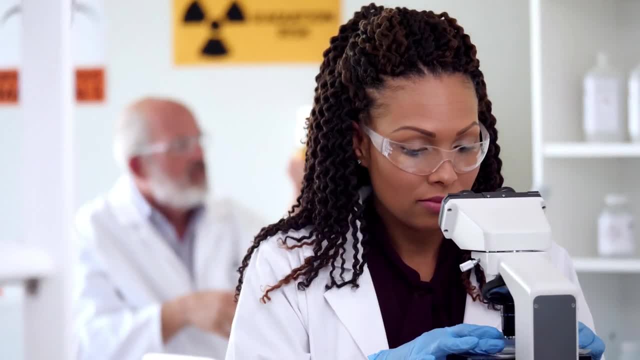 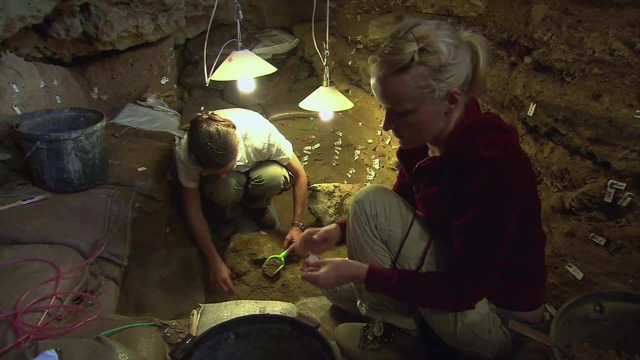 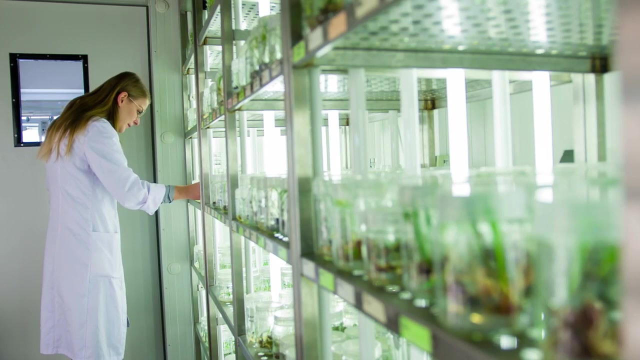 Science-related occupations account for over one million jobs. Social science occupations include political scientists, economists, anthropologists and archaeologists, while life and physical scientists include biologists, biochemists, park naturalists, hydrologists, geologists and physicists. 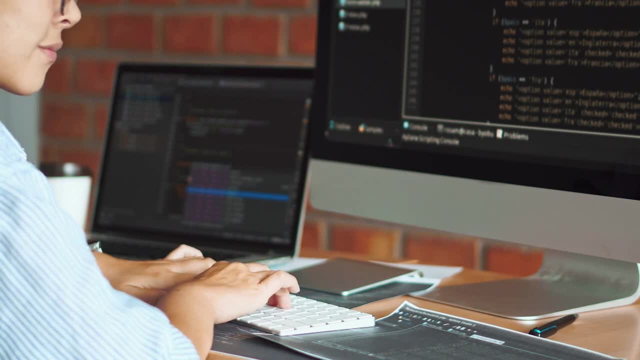 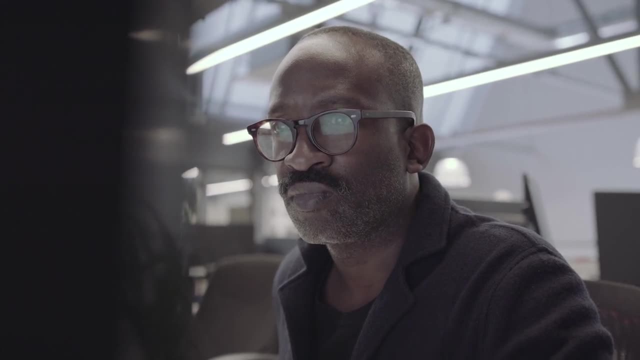 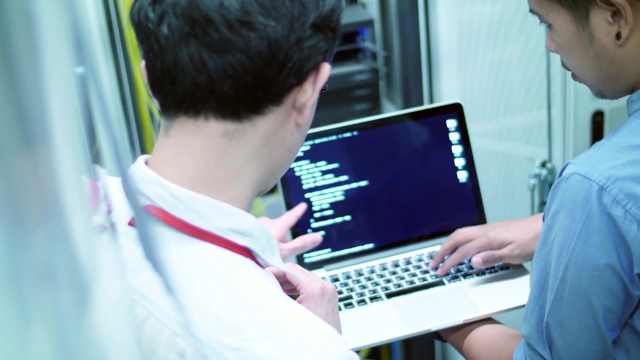 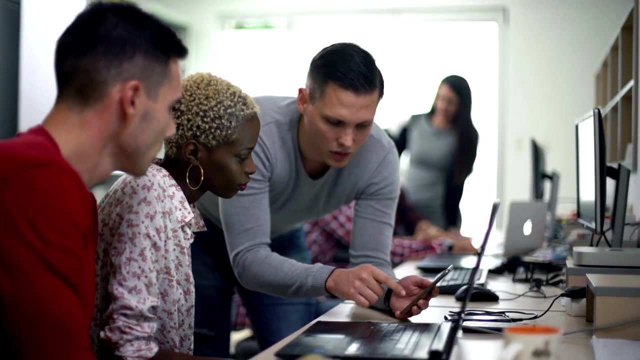 The technology sector employs the largest number of STEM workers in many fast-growing fields. Some require technical training or an associate's degree, such as web developers, computer user support specialists and computer network support specialists. Other IT fields require a bachelor's degree, including computer systems analysts, software. 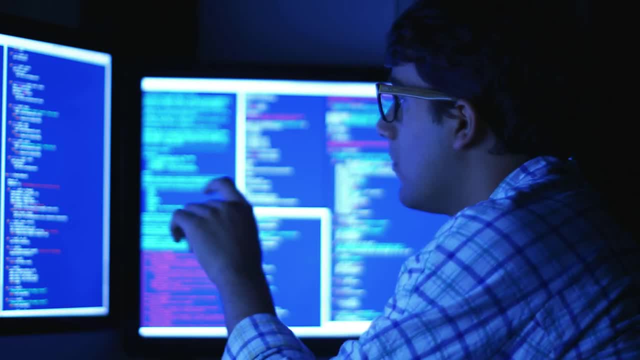 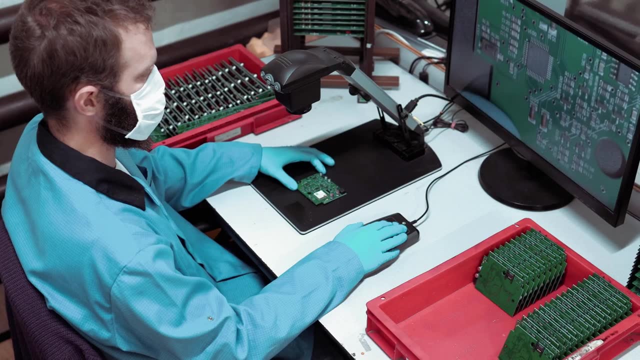 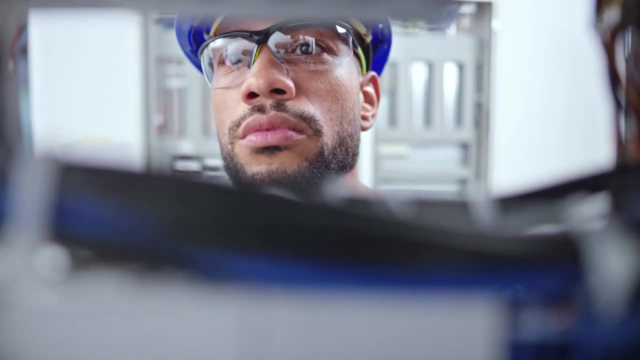 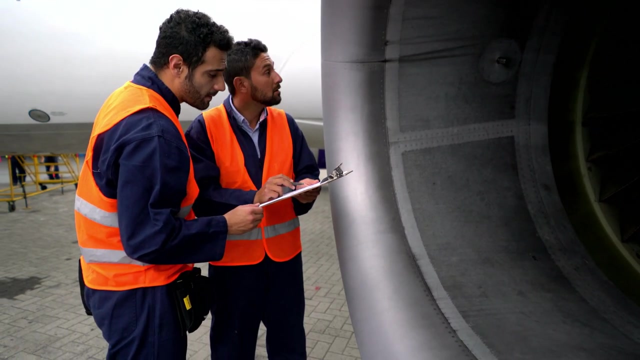 applications developers and information security analysts. Engineering fields at the associate's degree level include electrical and electronics drafters, civil engineering technicians and engineers. A bachelor's degree is needed for civil electrical and mechanical engineering, as well as the less commonly known engineering fields in aerospace, biochemical energy. 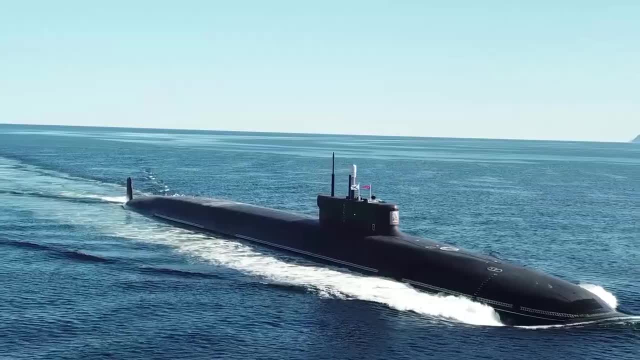 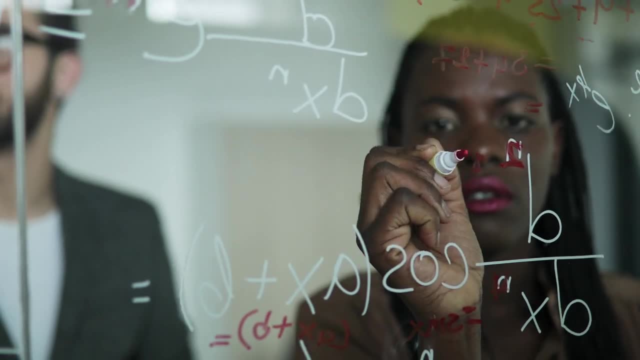 industrial, robotics, marine engineering and naval architecture. The mathematics sector employs fewer people than other STEM areas and requires a bachelor's degree for entry into almost any occupation. The bachelor's degree is required for engineering, engineering and mechanical engineering. The bachelor's degree is required for engineering, engineering and mechanical engineering. 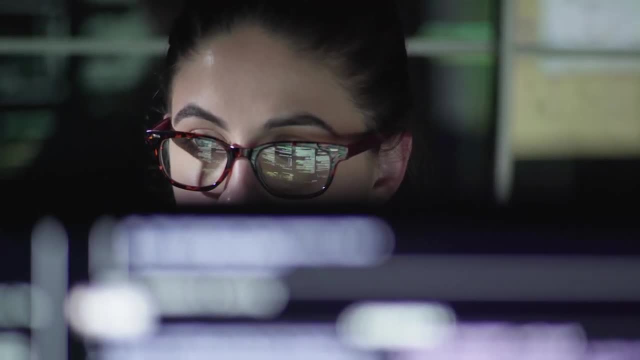 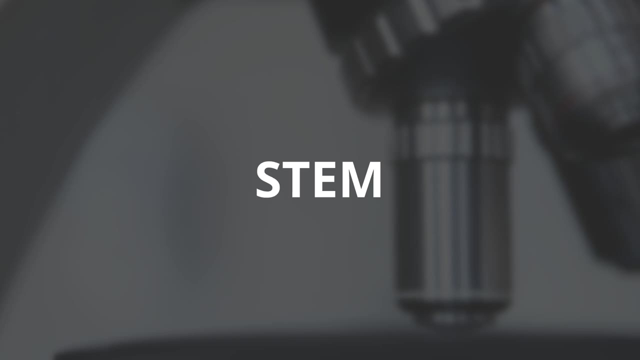 The bachelor's degree is required for engineering, engineering and mechanical engineering. Jobs as mathematicians, statisticians and actuaries are among the fastest-growing occupations in the entire career cluster. Is a career in science, technology, engineering and math for you.